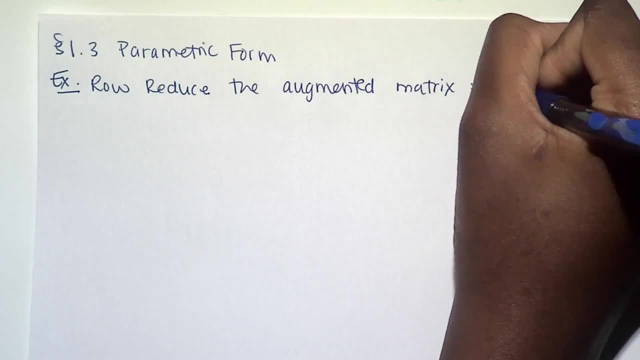 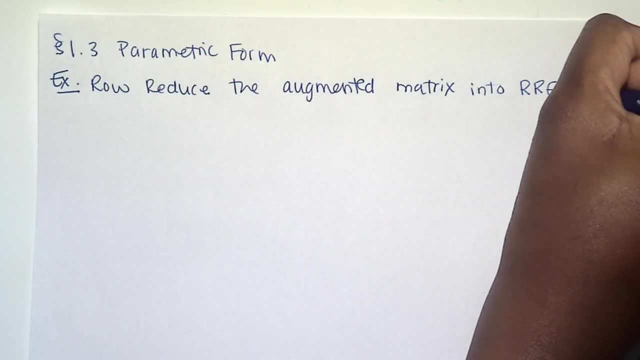 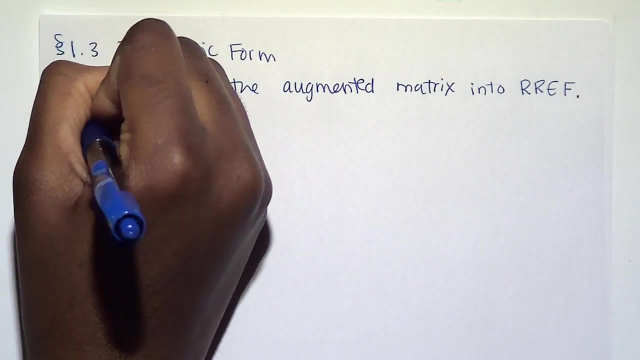 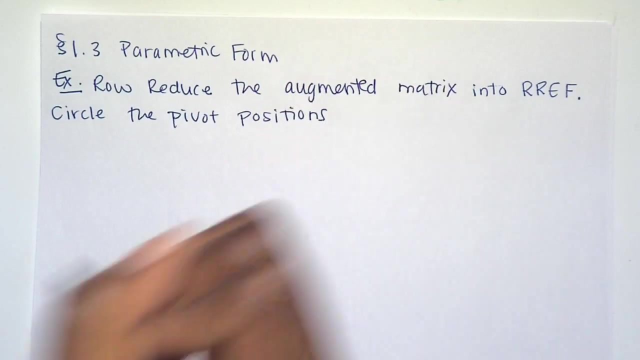 Into R, R, E, F. So reduced row, echelon form, And then, after we've done that, we are going to circle the pivot positions In the final circle. we're going to circle the pivot positions In the final circle. we're going to circle the pivot positions. 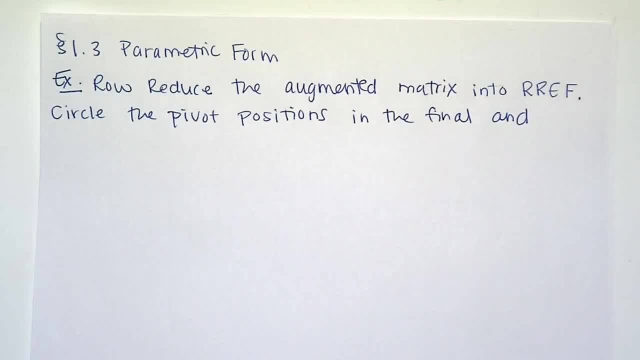 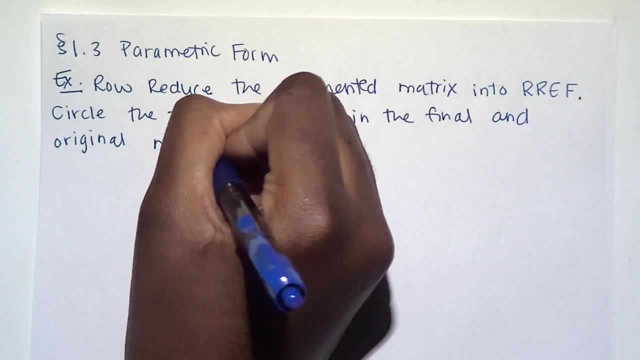 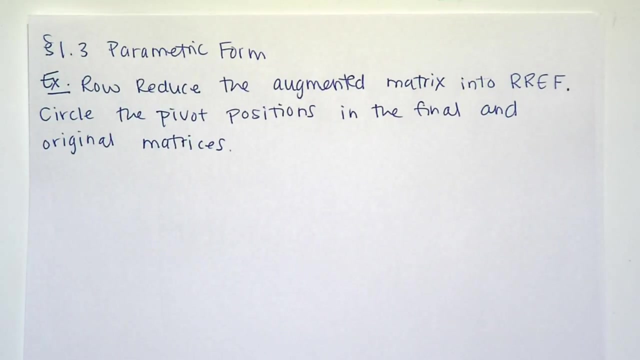 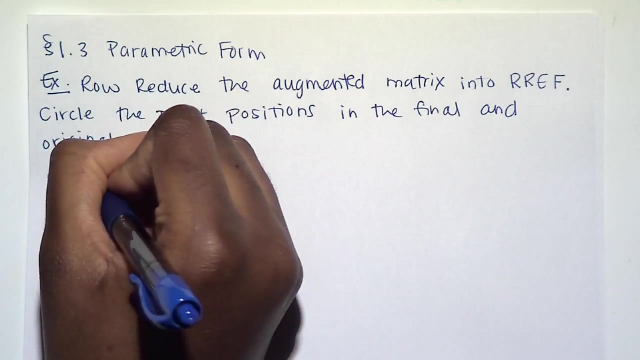 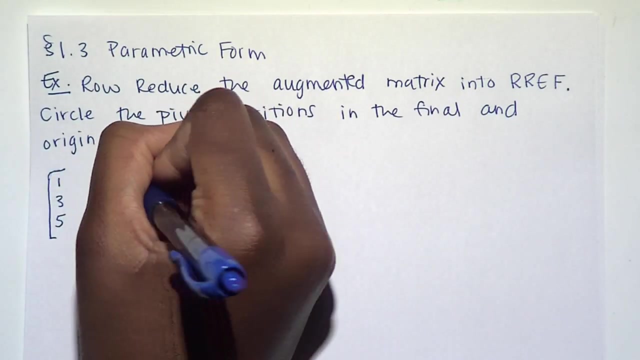 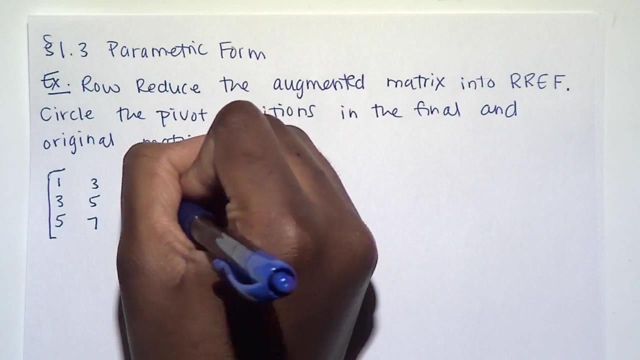 So we're going to row, reduce the augmented matrix into R, R, E, F and circle the pivot positions in the final and original matrices. So here is our augmented matrix that represents a linear system. So I'm going to go down the columns 1, 3, 5, 3, 5,, 7, 5,, 7,, 9, and then our system is going to equal 7,, 9,, 11.. 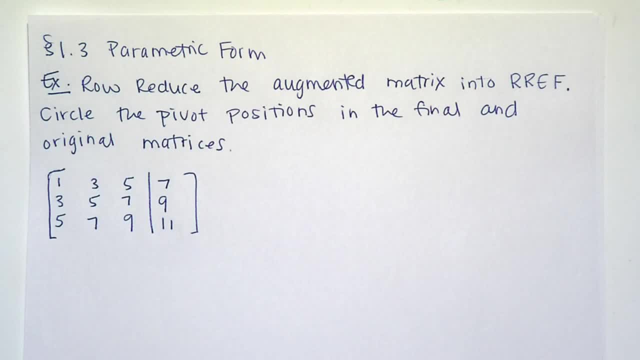 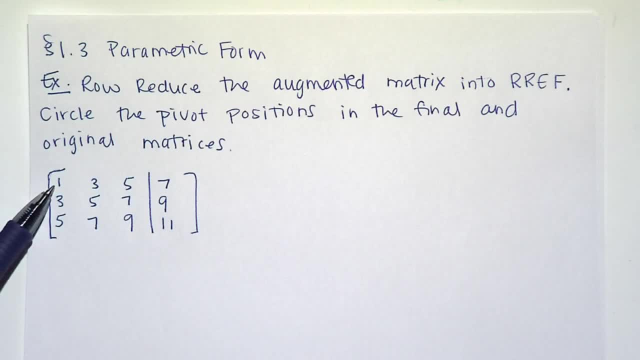 So I'm going to go down the columns 1,, 3,, 5,, 3, 5,, 7,, 9, and then our system is going to equal 7,, 9,, 11.. position up here, and I see that it's already a one. So we are good to go. I can use this. 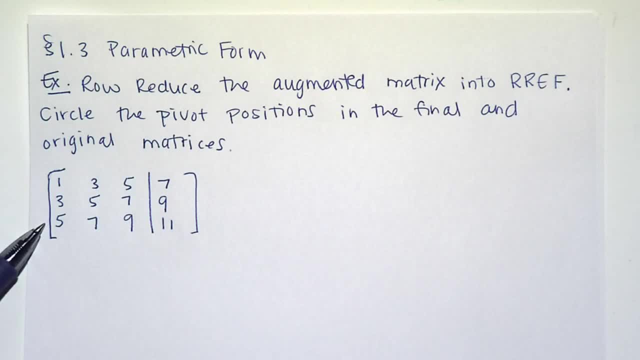 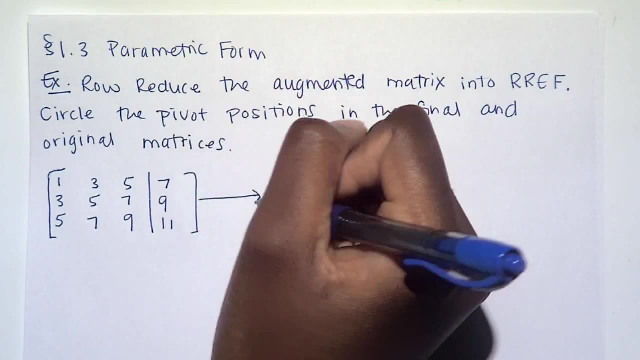 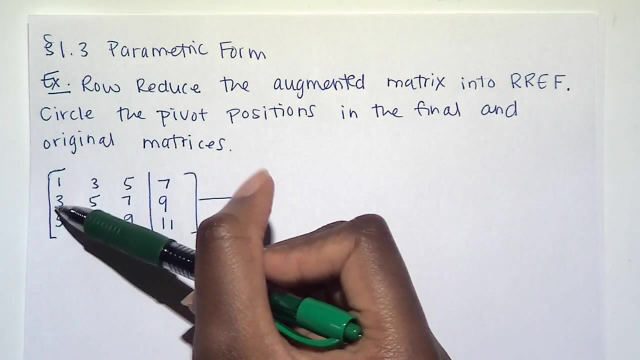 one to eliminate the three and the five, And so when you are row reducing, it's really important that you show which row operations you're using. It makes it much easier to grade and give you partial credit. Okay, So I want to update row two and turn it into a zero. 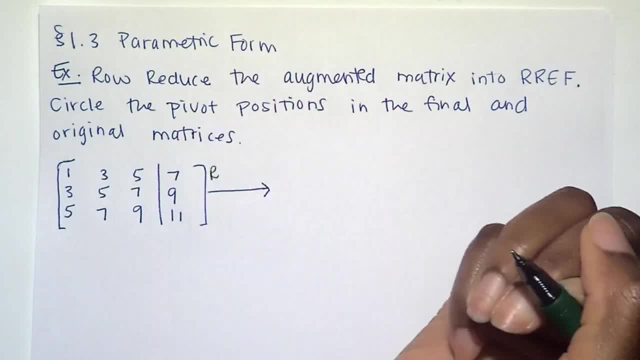 So the way I like to do this- you'll see it in different ways, but just make sure you're clear in your notation- I want to update row two, So get a new row two. So I like to call it row two prime. And the way I'm going to do it is I'm going to multiply negative three. 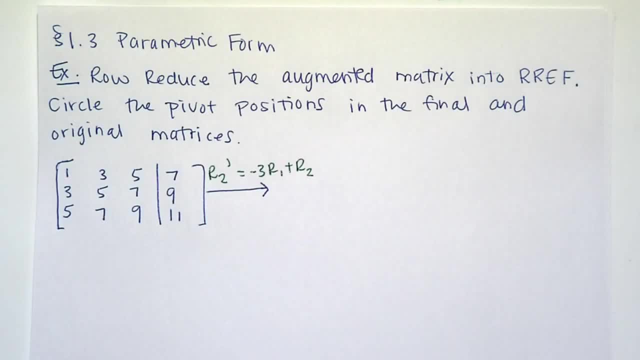 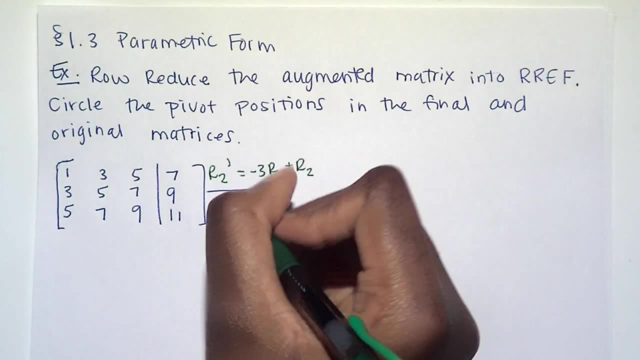 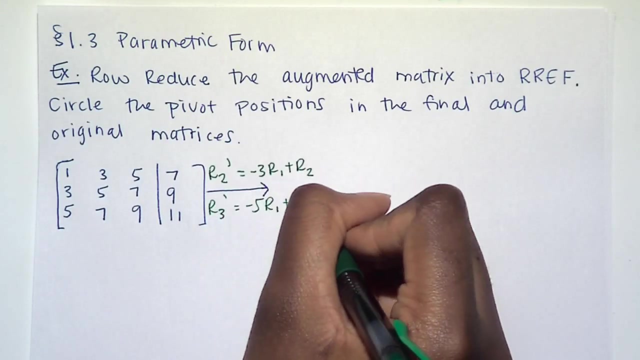 times R1 and then add it to R2.. And since I'm working with the same thing below this one, I can do it in the same line: update R3, the third row, by multiplying negative five times R1 and add it to R3.. And you know you've done it right if you get zeros under. 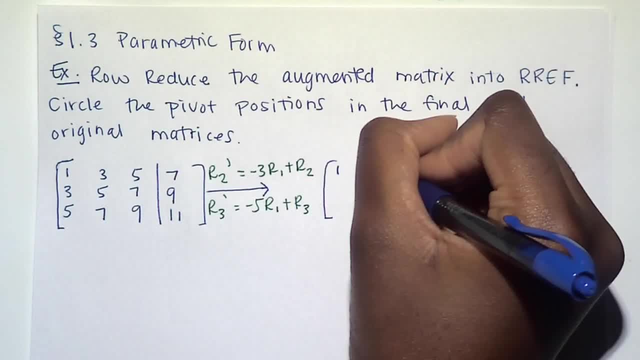 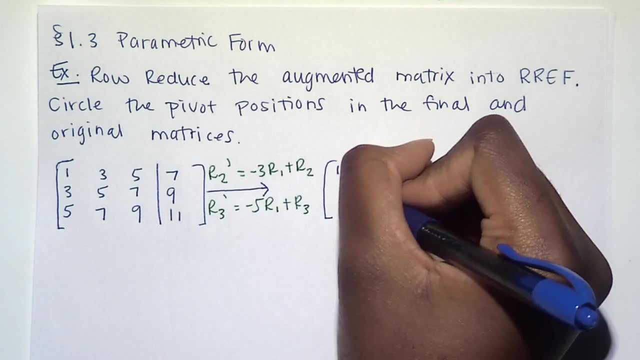 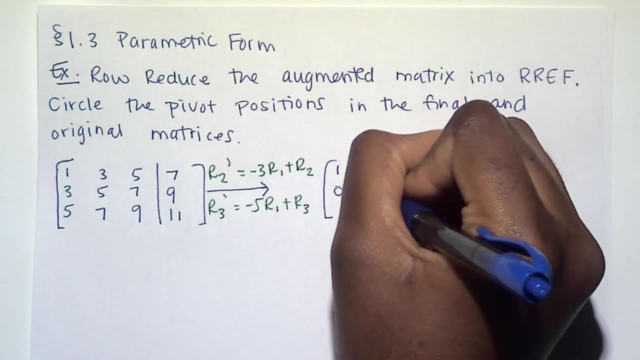 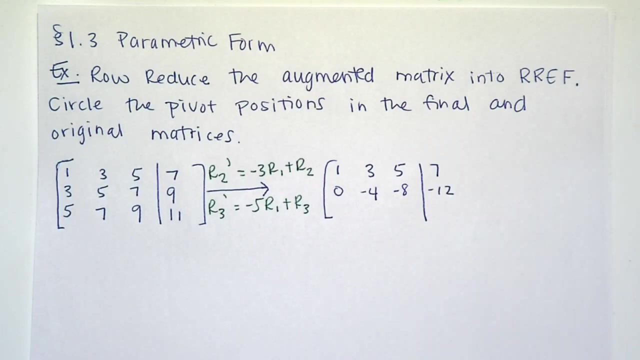 here. All right, So the first row is going to stay the same because we have not updated it. We should get a zero here, a negative four, a negative eight, a negative nine, a negative 10.. All right, And feel free to pause this to do the math on your own, just to make sure. 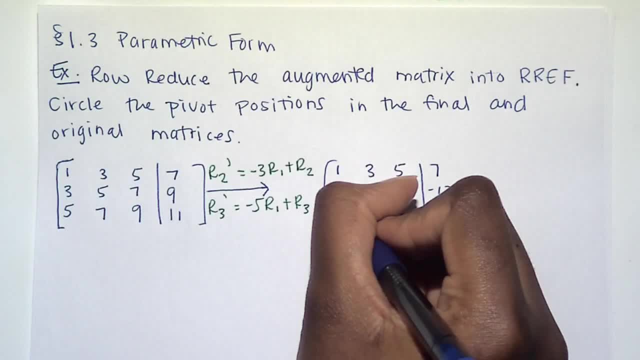 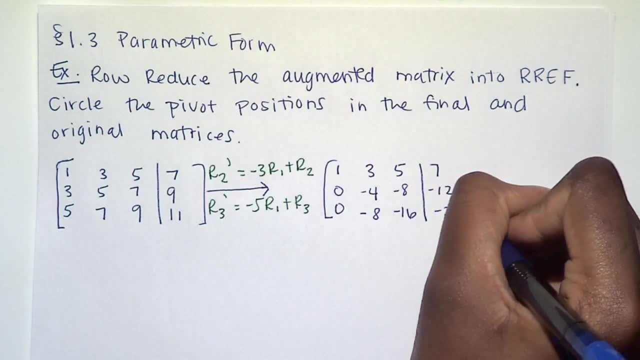 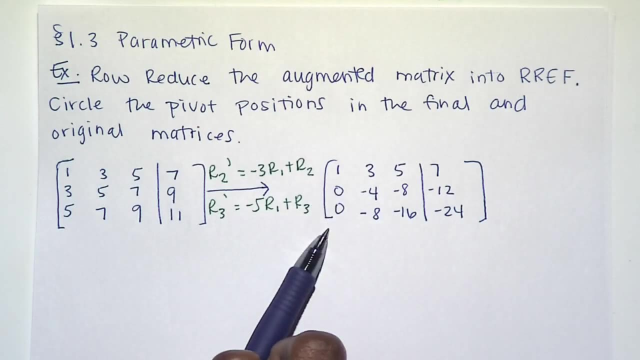 that I'm correct and that you can do this on your own With zero negative eight. negative 16, negative 24.. Okay, All right, So I have all zeros below this one. I'm going to move to the next diagonal piece, which is this negative four. It is not a one already, So 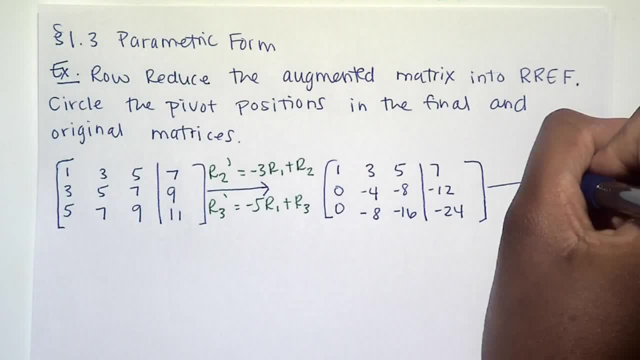 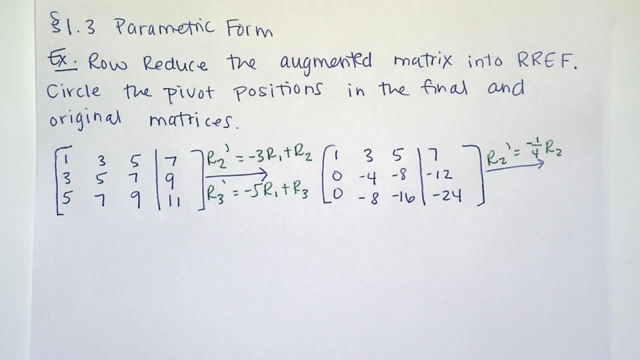 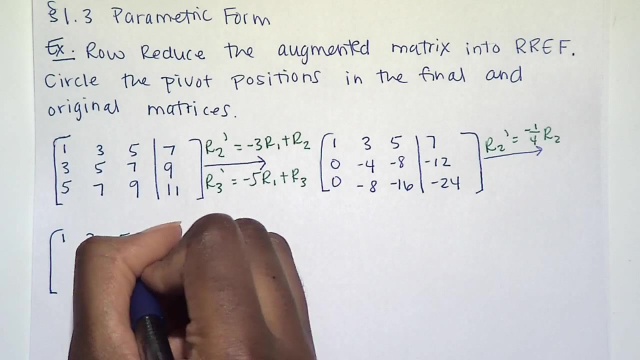 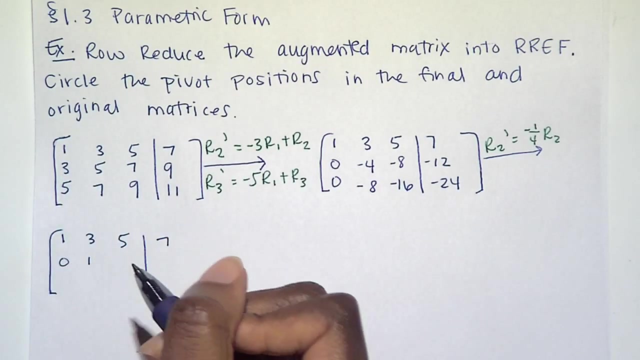 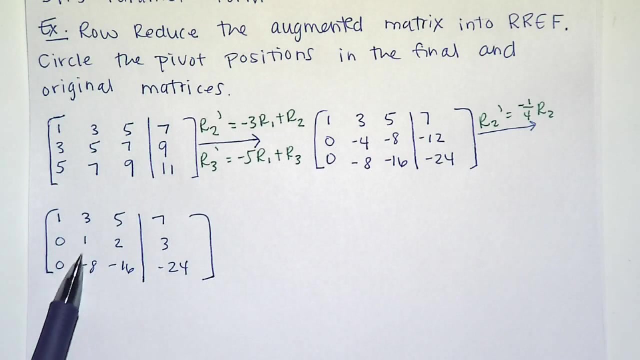 I need to scale it and turn it into a one So I can update my second row by multiplying one fourth times it All right, so everything will stay the same except row two. All right, So now I have this one that I can use to pivot So I can turn everything below it into a zero. 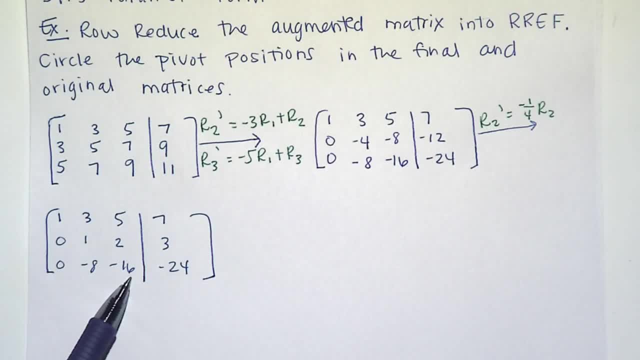 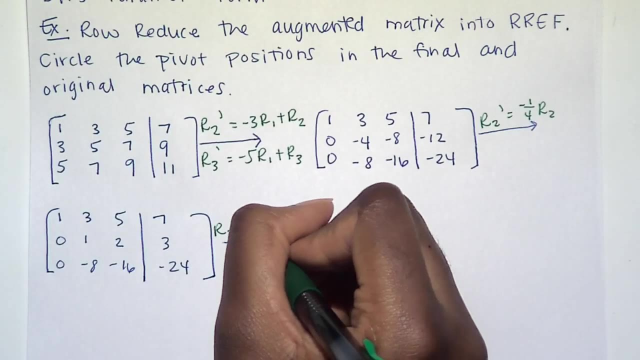 So you want to make sure you do everything below, first to go into REF and then come back and get the top numbers. Okay, So, So I will be updating row three And to do that I'm going to multiply eight times R2. 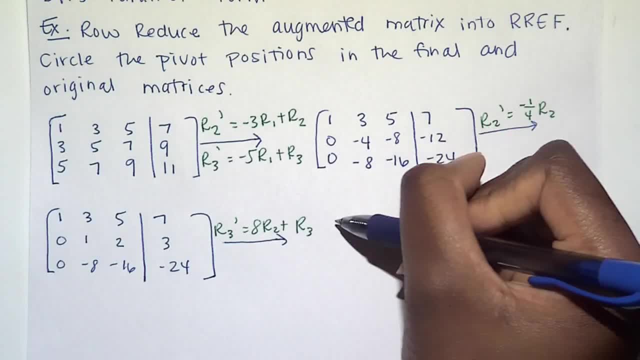 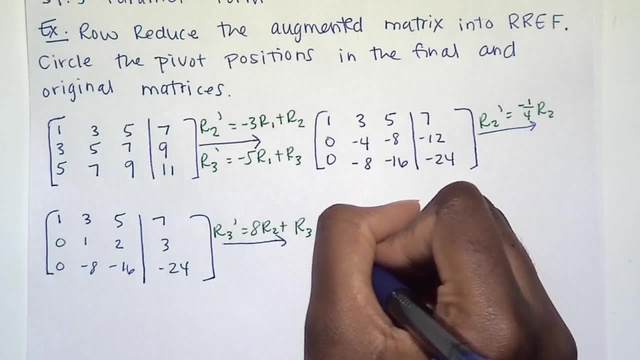 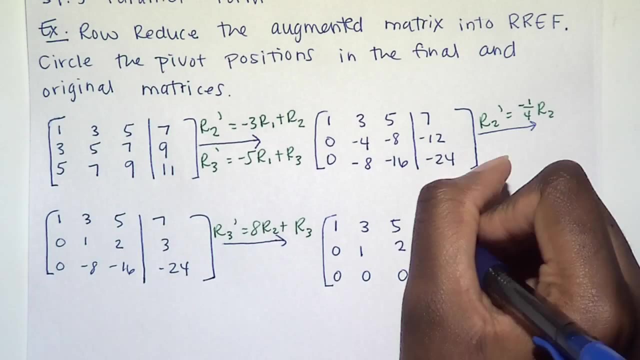 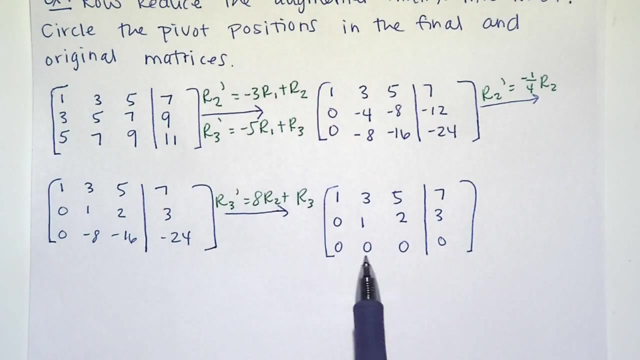 and add it to R3.. Okay, So notice, we're going to have all zeros in the bottom and that's okay. but that just tells us we're not going to have a third pivot position because where there's no way that we can use a zero to update these numbers up here. But notice, we are now in REF, So 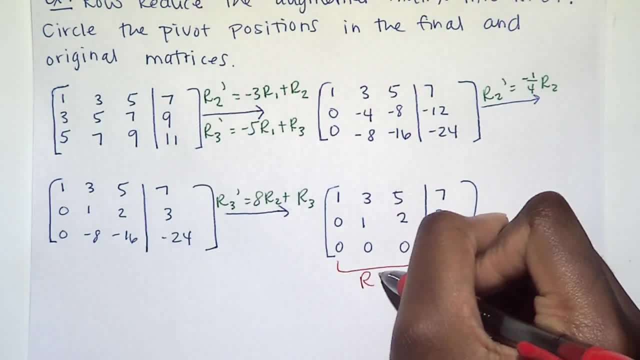 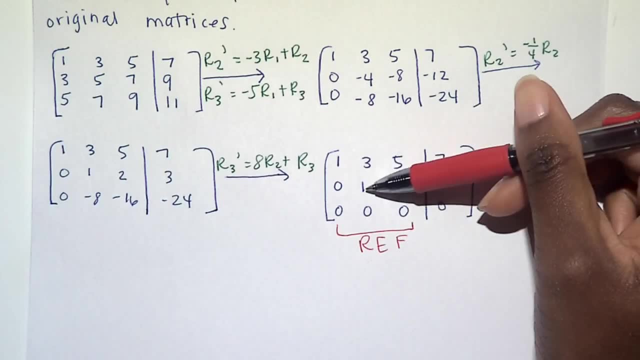 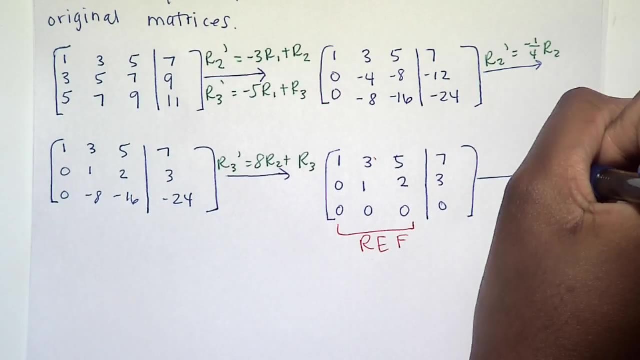 remember, our first goal is always to get it into reduced echelon form or row echelon form. Alright, so now we can use this pivot position to get rid of this 3 and I think we'll be good to go. So I'm updating row 1 by multiplying negative 3 times the second row and adding it to the 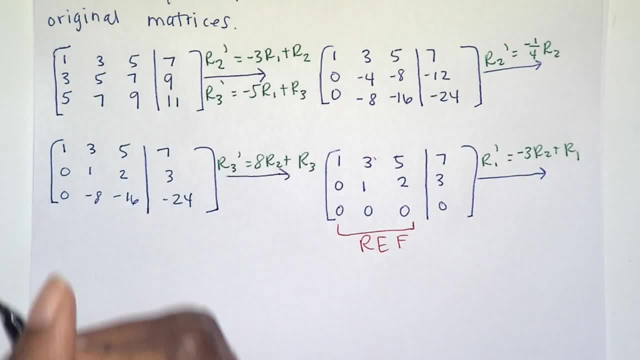 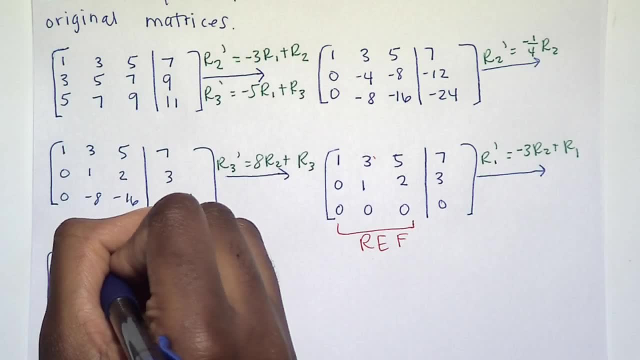 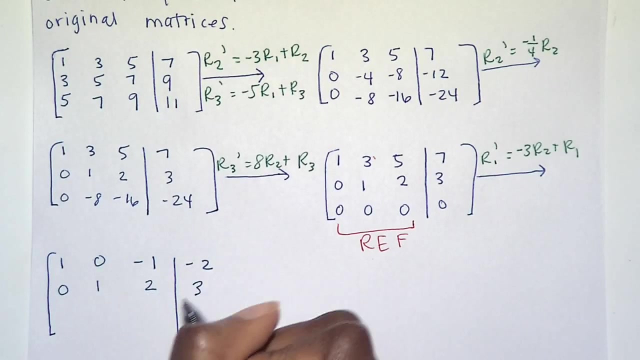 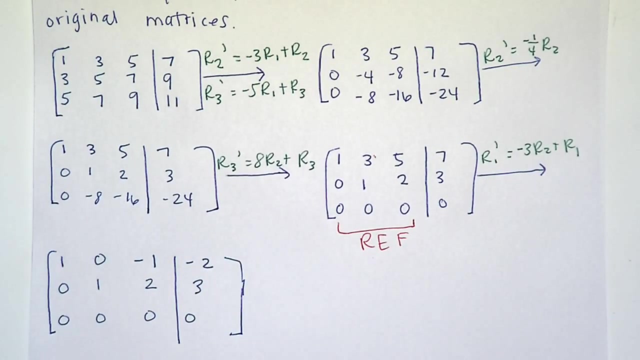 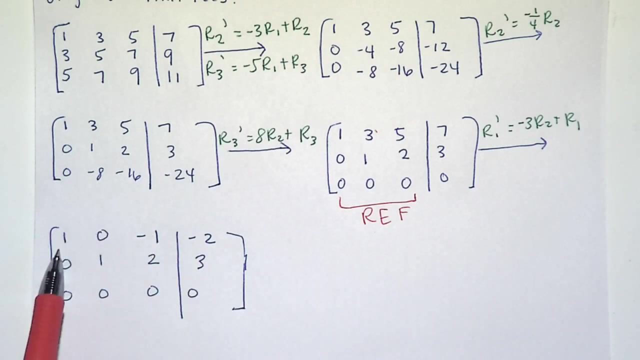 first: Okay, so this is what I'm getting. Everything else should stay the same. Okay, Okay, All right, and so now, if you notice, we have 1s in the diagonal as much as we could. We have 0s below them, but also we have 0s above, so that means we are in RREF reduced. 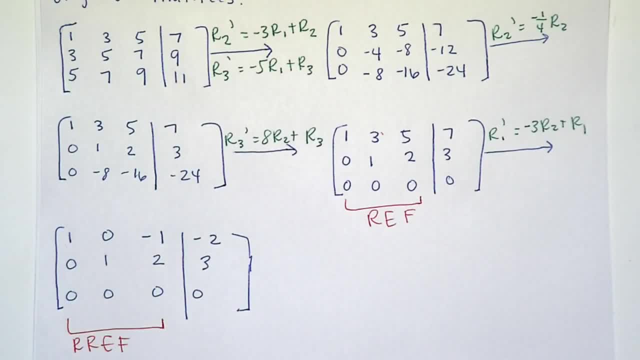 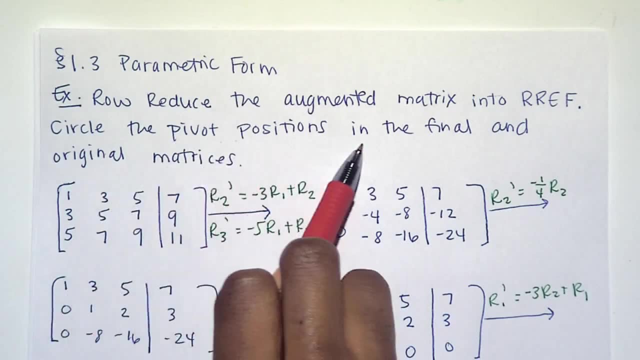 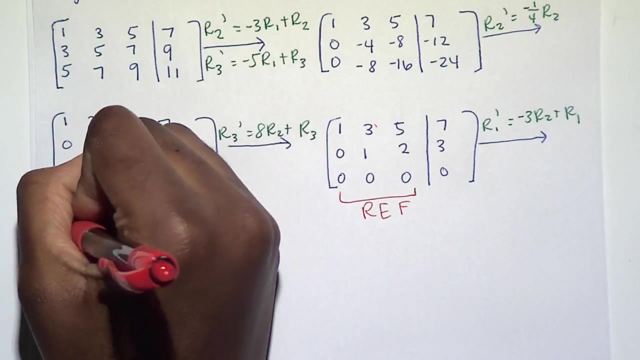 row echelon form, which is exactly what our goal was. So the next thing that we were asked to do is to circle the pivot position. So we have two pivot positions in the final and original matrices. so we can use the final to see: oh, we have two pivot positions, the first and second diagonals, and they are going. 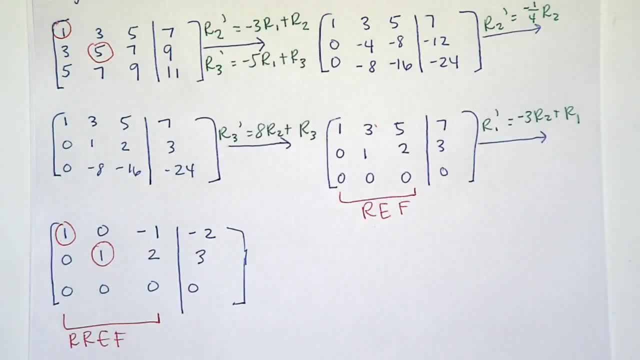 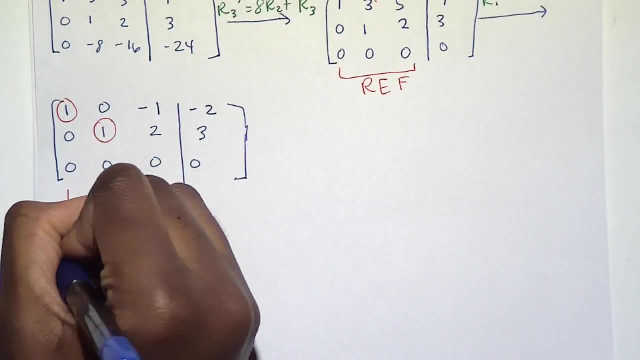 to correspond to the 1 and the 5 in the original augmented matrix. Okay, so the final thing that I want us to do with this example is to find the solution. All right, So let us find the solution, Okay, Okay. 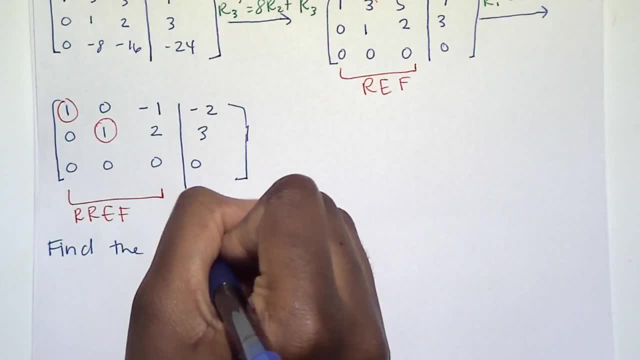 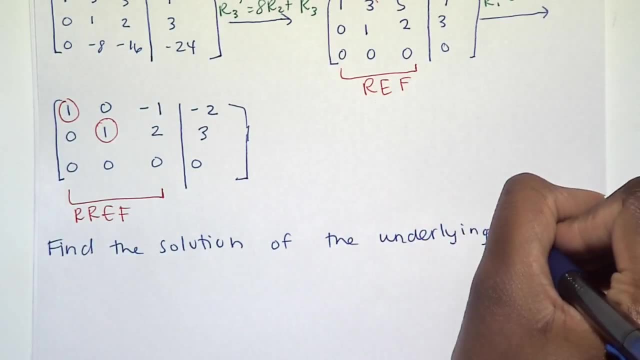 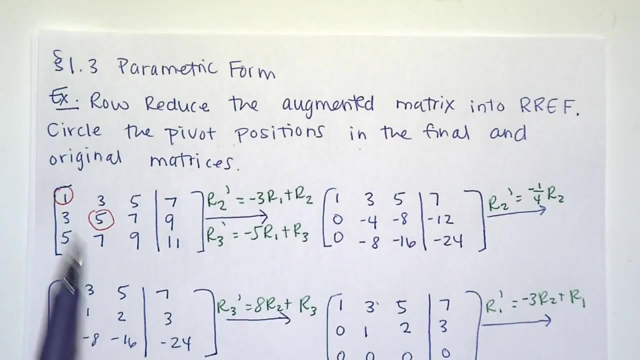 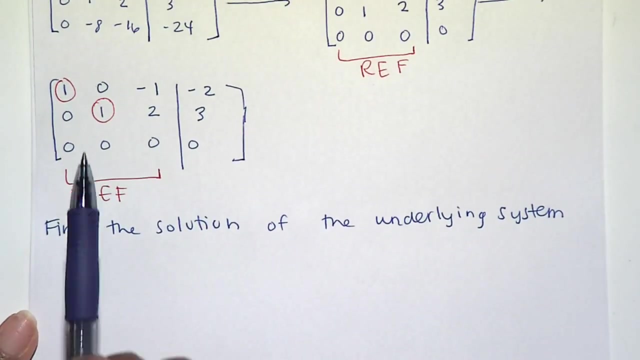 So let us find the solution of the underlying system, and so I actually want us to write out the system first, and so, yes, you could write the original system from the first augmented matrix. However, it's so much easier to solve with the reduced one right. 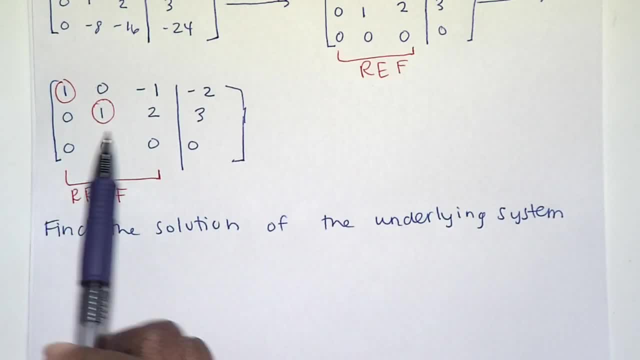 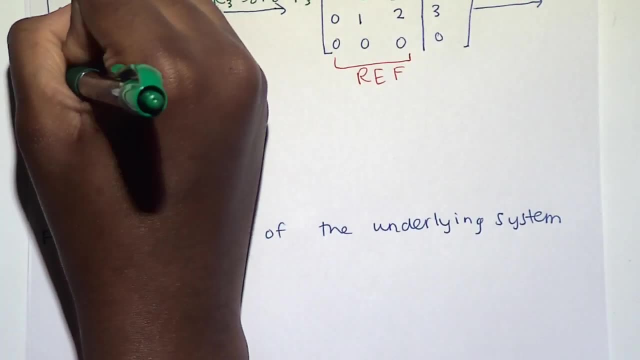 We know these are row equivalent, so we can just use this. All right. so the first, if we look at the first line, remember, so something to keep in mind. the first column represents the variable x1,, second column, x2, and x3.. 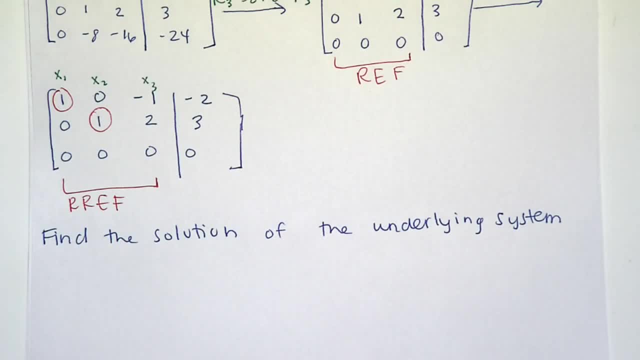 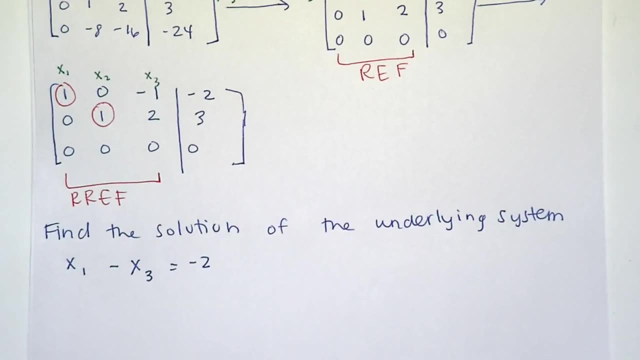 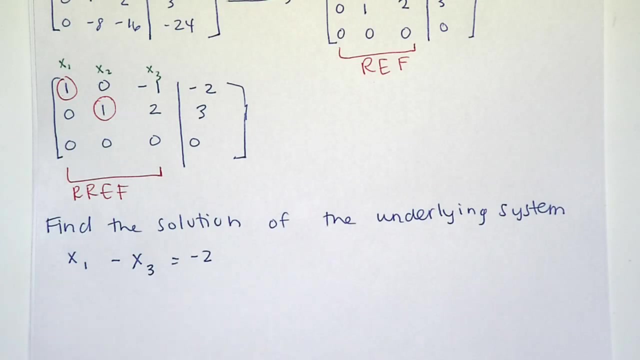 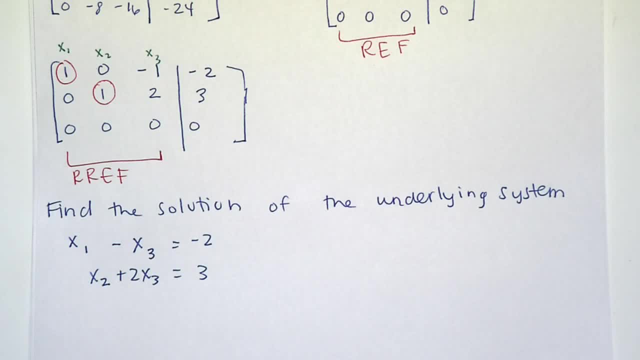 Okay, Also for the second row, we see that x2 plus 2x3 equals 3,. and then the third row. we have all zeros. We don't have to use it. I won't be writing it down in the future, but I'm going to write it down today: 0x1. 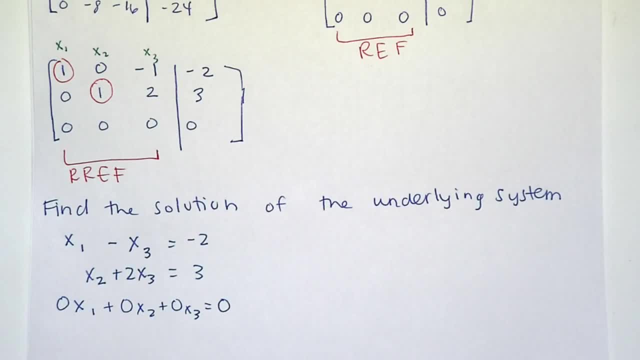 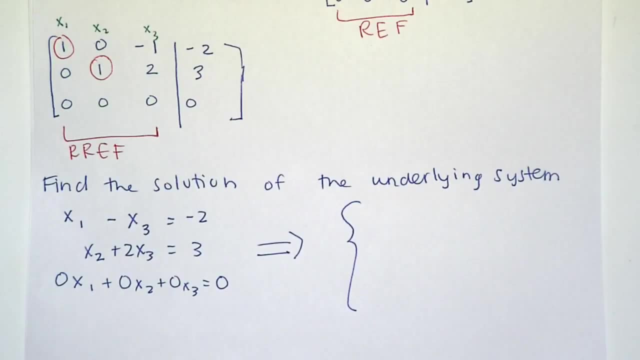 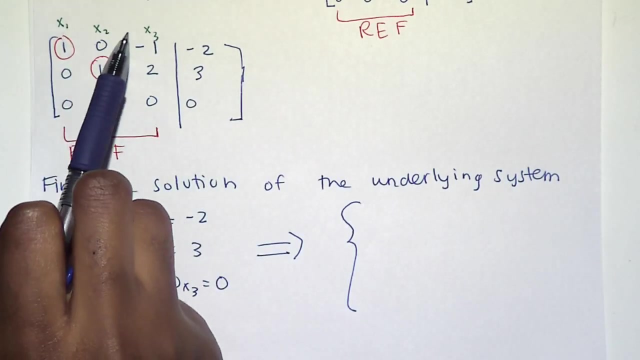 plus 0x2 plus 0x3 equals 0.. All right, let's get into the system. I mean the solution. like to do a curly brace to write out my solution and remember our solution is going to be x1,, x2, and x3. So I'm going to take each one of these. So take the. 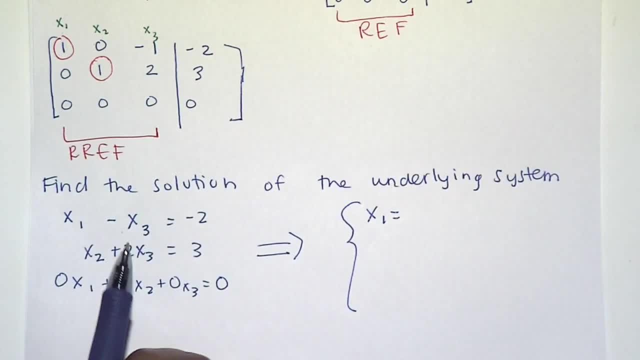 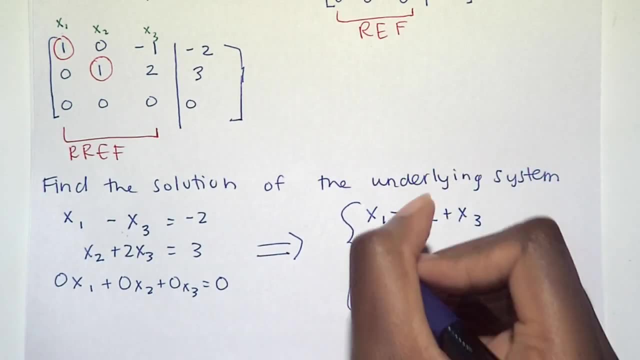 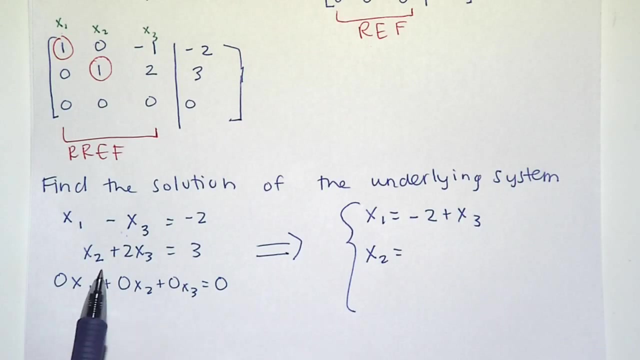 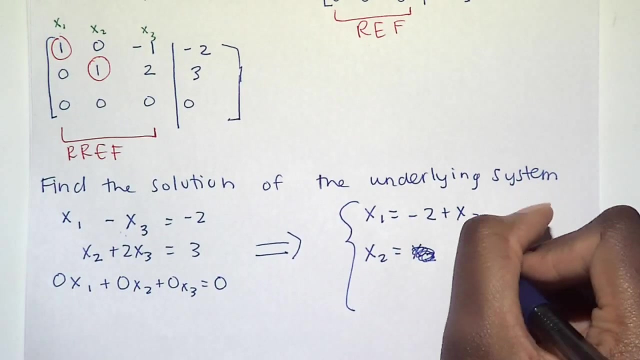 first equation and solve for x1, and I can do that by moving the x3 over. In the second equation, I'm going to solve for x2, which I'll do by moving this part over. Well, this should be 3, plus 2, plus x3, and